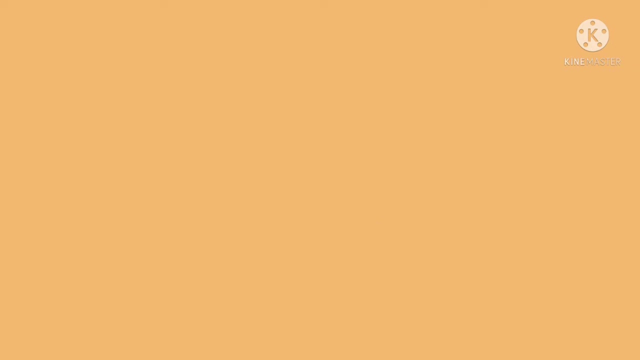 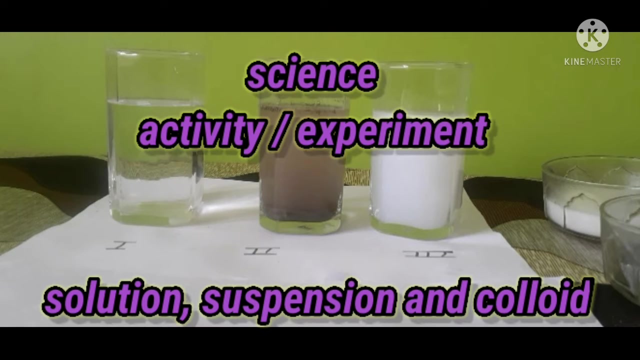 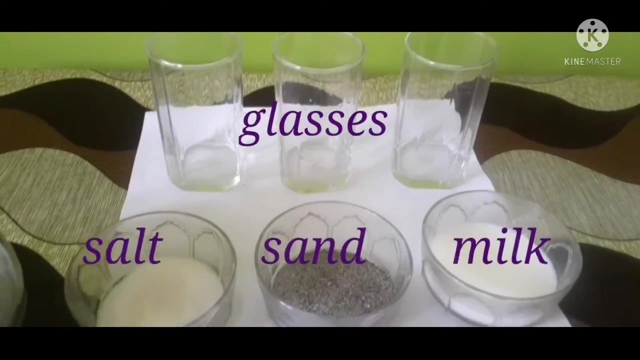 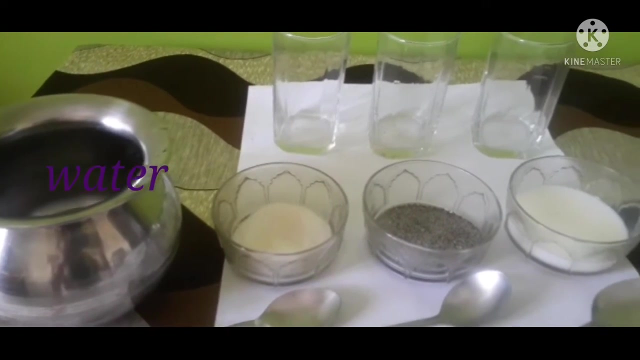 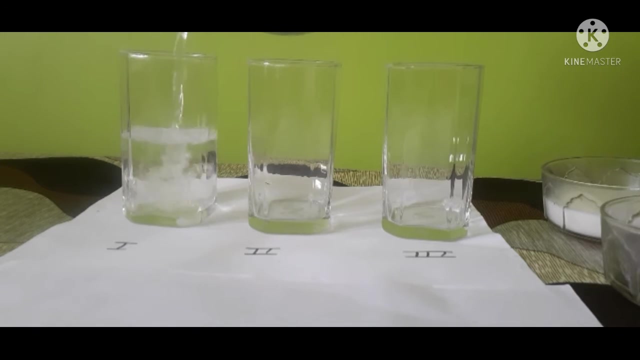 hello everyone, welcome to my channel. today we are doing an experiment showing difference between solution, suspension and collide. so for this experiment we require some material: three glasses, some salt, sand and milk and some water. well, let's start the experiment. we take water in glasses now. in first glass we add some salt. 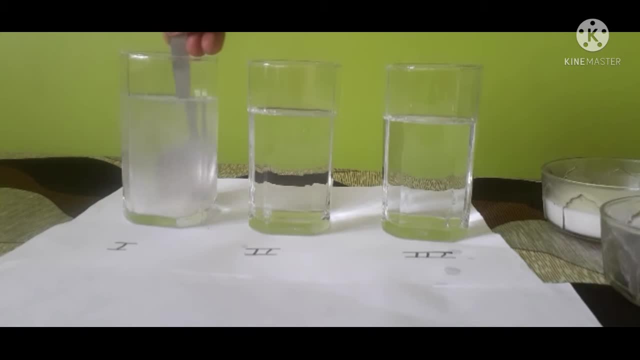 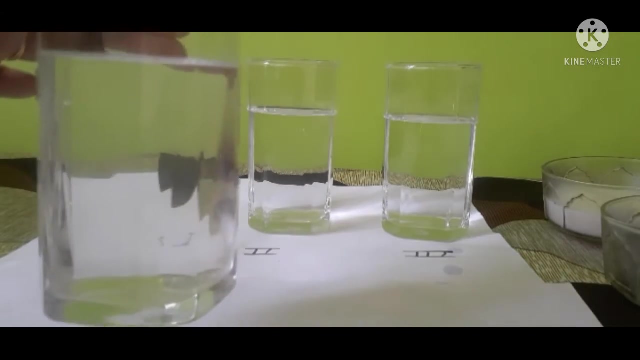 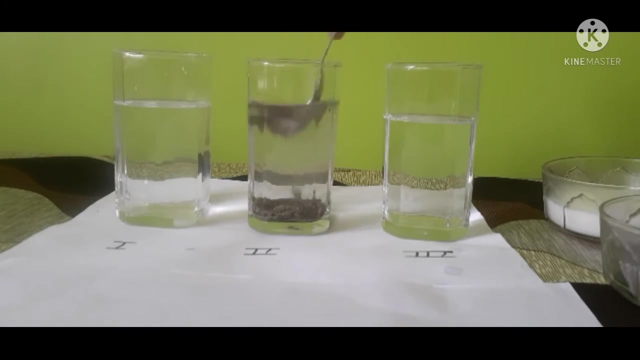 stir it well with spoon. we can see salt dissolved completely water and finally we get a clear, transparent solution of salt. in second glass we add some sand or soil. stir it with the spoon. we can see easily that sand particle does not dissolve in water. we can see that sand particle does not dissolve in water. 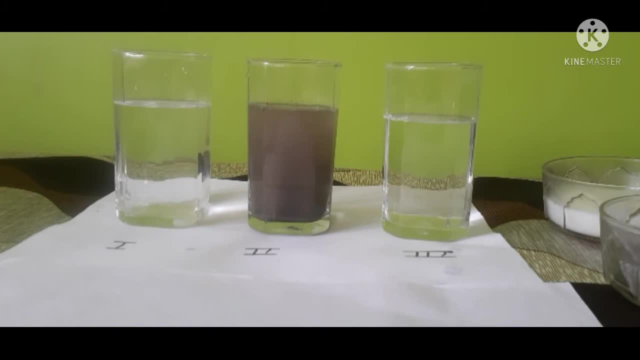 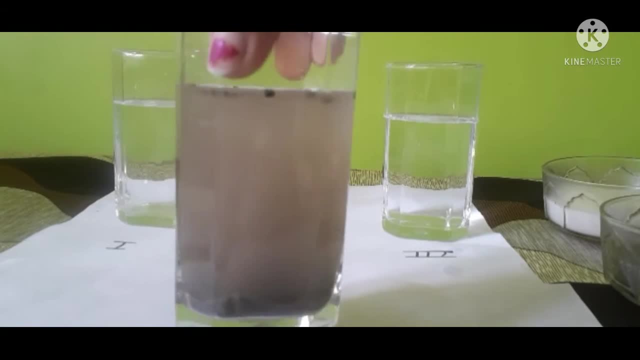 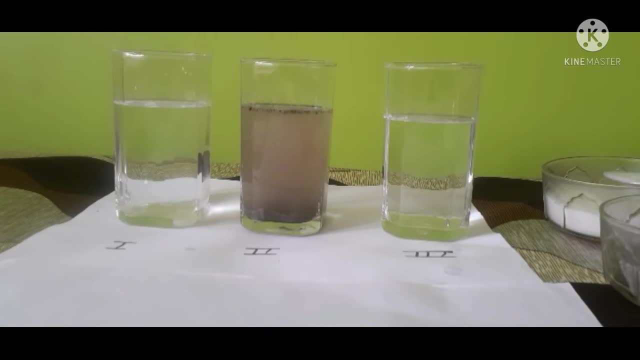 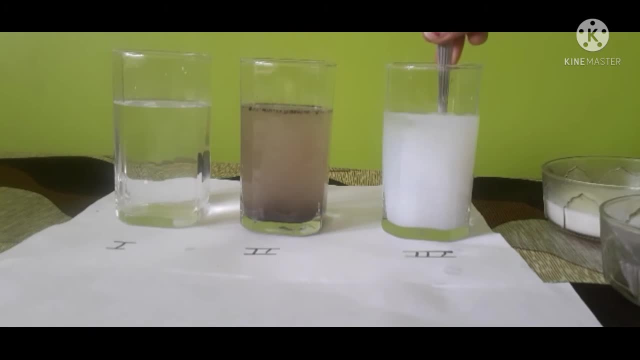 Stir it well with the spoon. Milk mix easily with the water. This is a colloid solution: milk colloid solution. Now, if we observe this salt solution, we can see that it is clear, transparent and homogeneous. We cannot see the particles of sand in it and this solution is stable also. 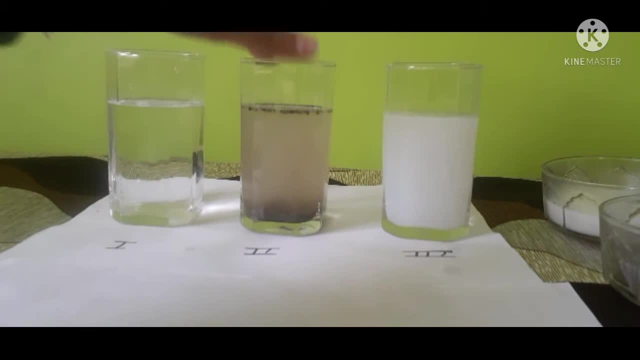 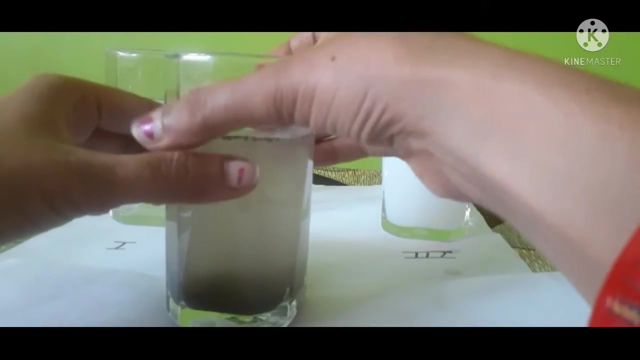 It means salt particle does not separate on standing. Now observe this suspension of sand. This is a heterogeneous mixture and we can easily see the sand particles in it, Sand particles settled at the bottom of the glass. It means the suspension of the glass. 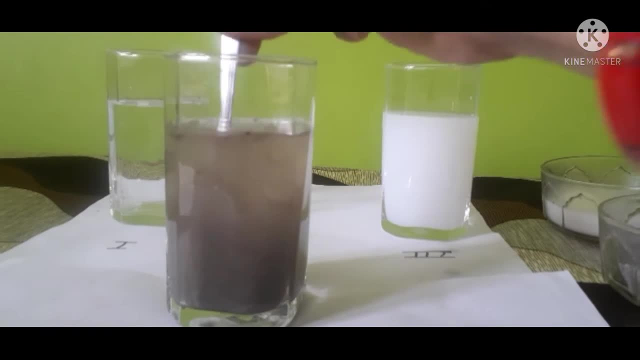 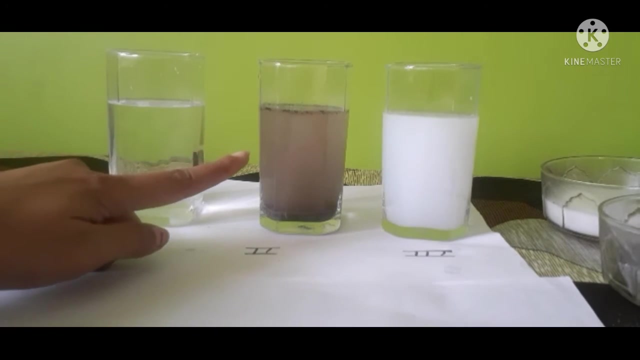 The suspension is not stable If we stir it. they suspended in water and after standing they settled at the bottom. We can separate easily the sand particles by the filtration process In milk colloid solution. we observe this is a translucent and homogeneous mixture. 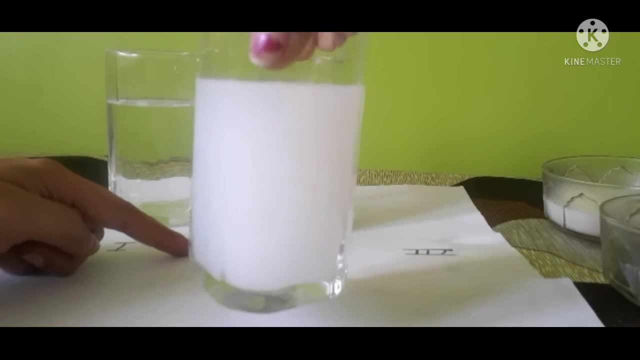 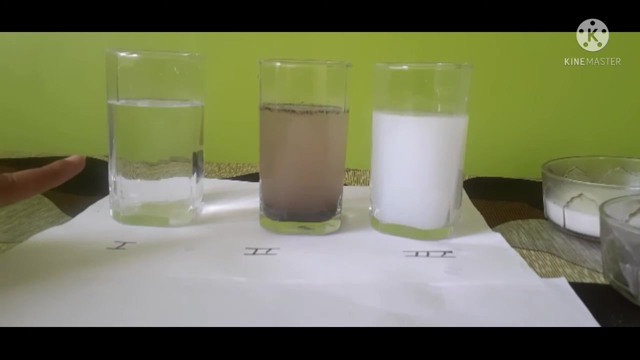 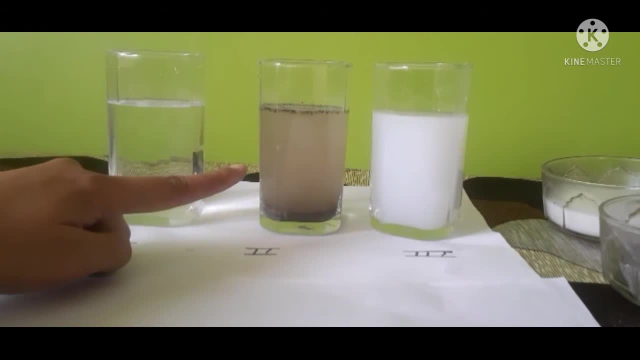 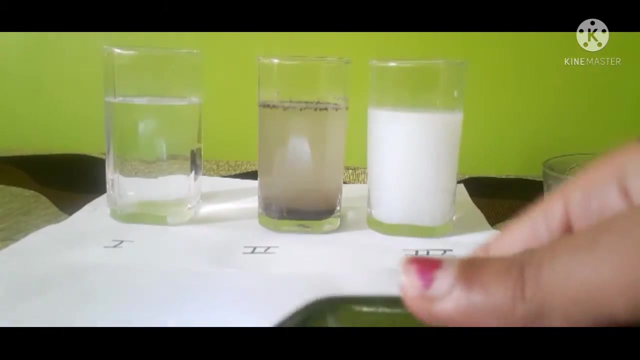 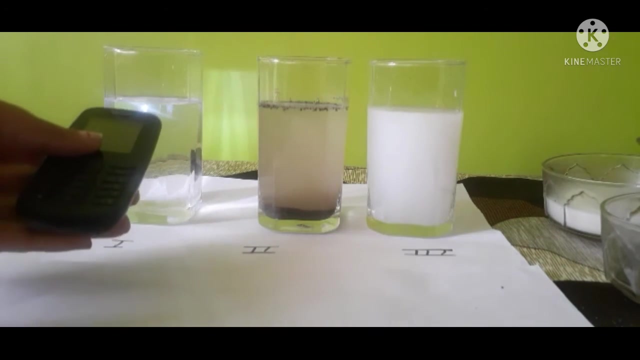 We cannot separate these particles by filtration, But in suspension particle size is large and we can separate easily by the filtration process. Now we pass light through this solution with our mobile phone, or we can use torch or laser light, etc. First we pass through the true solution. 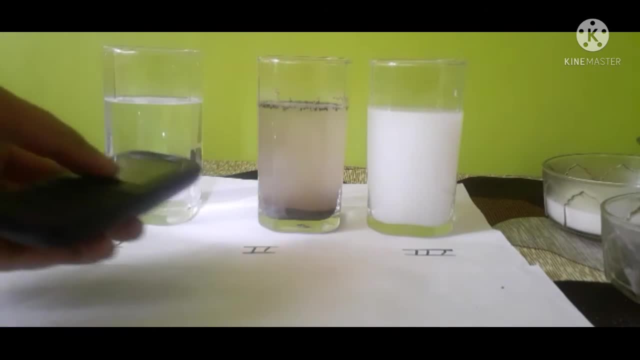 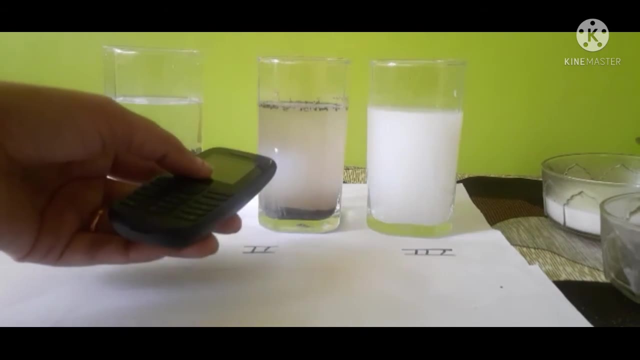 We can easily see that light passes through it, but there is no scattering. While passing the light through the suspension, it also passes through it and there is no scattering. While it passes through the suspension, it also passes through it and there is no scattering.